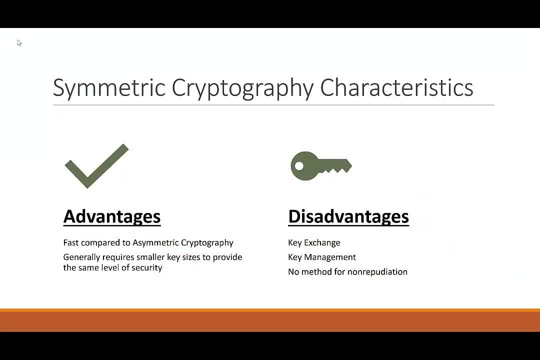 Here are some of the characteristics of symmetric cryptography. So some of the advantages are that symmetric cryptography is fast, especially when compared to asymmetric cryptography, And generally requires smaller key sizes to provide the same level of security. For these reasons, symmetric cryptography is typically used for any sort of bulk encryption. 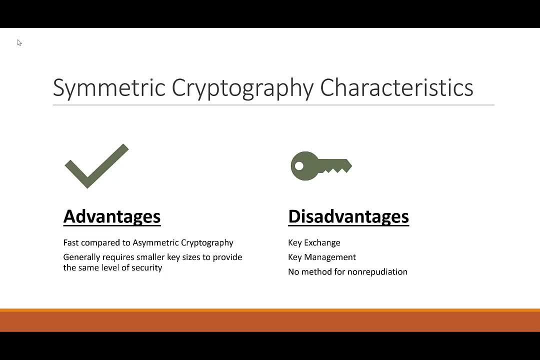 just due to the speed factor. Some of the disadvantages are: there is no real built-in method for key exchange. There's really no method for key management that's built in And also there is no method for non-repudiation. So the idea with non-repudiation is, if I were to 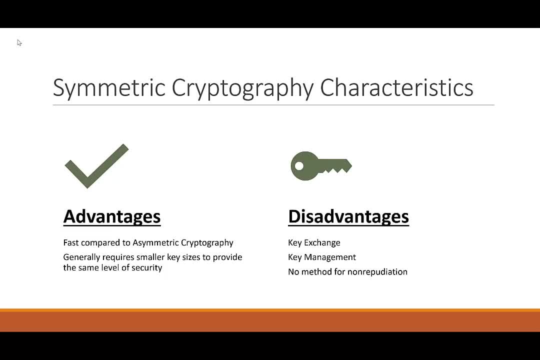 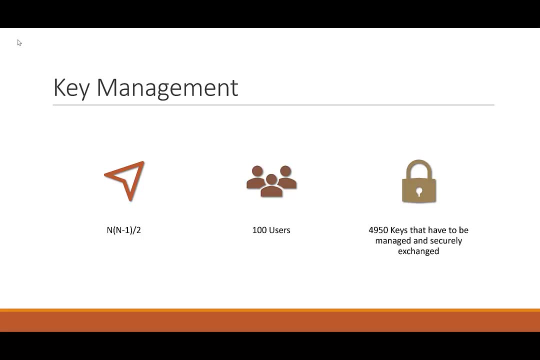 send an email to, let's just say, Alice, non-repudiation would prevent me from denying that I sent that email, And so that's a feature that's not available with symmetric cryptography. So key management is, like I said, a problem with Kerberos, And the idea here is in this example. 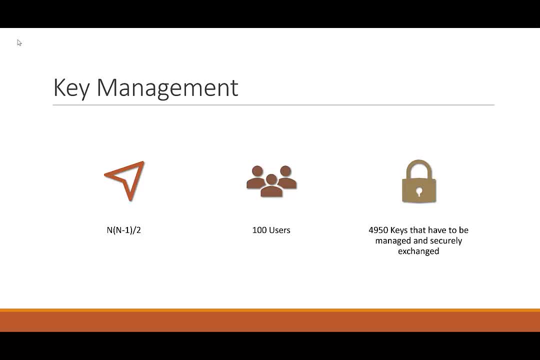 here. you can imagine an environment where you have a hundred users And if they were going to use symmetric cryptography to securely communicate with each other, each one of those users would have to have a unique key for each other person they were having a conversation with, So you would have 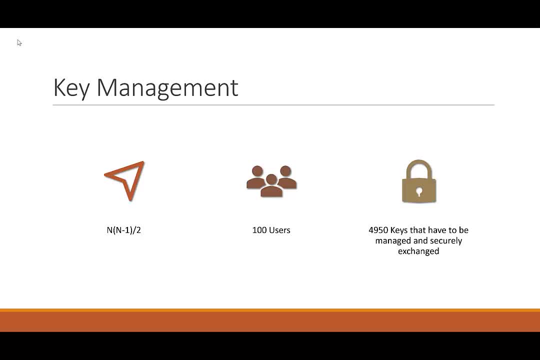 a lot of keys. In fact, you would have roughly around 5,000 keys if they were all sharing information with each other and trying to do that securely with symmetric cryptography. So that can be a problem. There are some solutions. So if we look at Kerberos, Kerberos uses symmetric 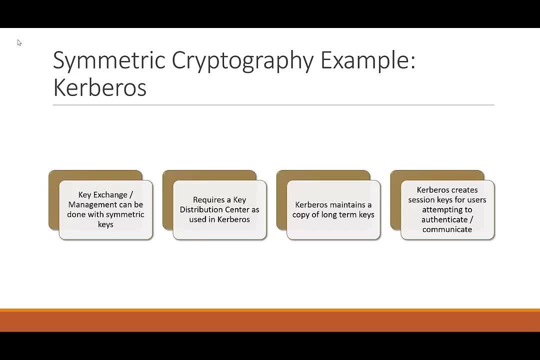 cryptography, but it does a good job of handling keys. There's long-term keys in terms of passwords. There's shorter, shorter keys that are used for, you know, different authentication sessions. So Kerberos definitely does do this. So Kerberos uses a key distribution center to handle most. 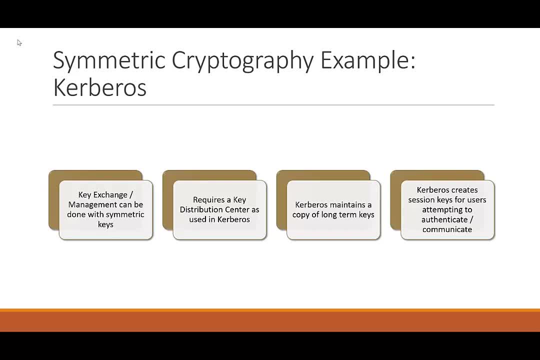 of this work And Kerberos does maintain the long-term keys, which are passwords, right Passwords for the machines, passwords for the users, that sort of thing- And Kerberos creates session keys for users when they're attempting to authenticate to. 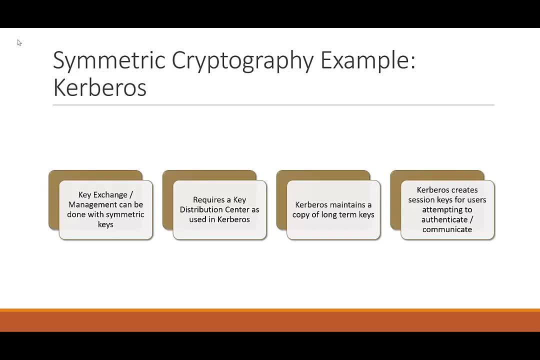 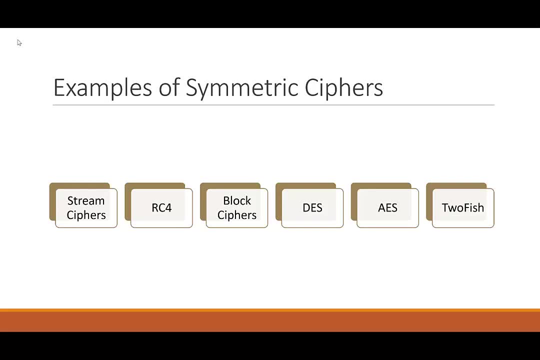 either the domain or to two different services in the domain. So again, just an example that Kerberos can handle this key management aspect. Some examples of symmetric cryptography are here, some different sort of algorithms. The most common one you typically see is AES, right. Some of the other ones you may not have heard of, but AES is a. 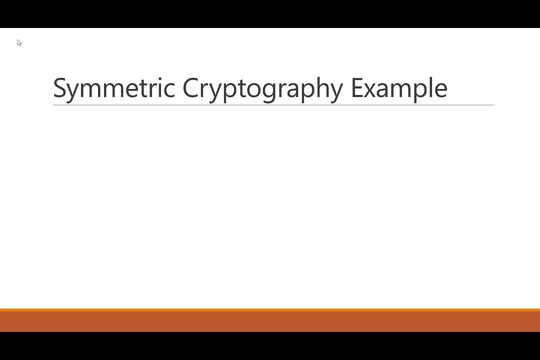 pretty common one. Here's an example of symmetric cryptography just to kind of illustrate how everything works. So in this example, Bob wants to encrypt data so that he can send the data securely to Alice. So what he does is he gets a copy of the data that he wants to protect. 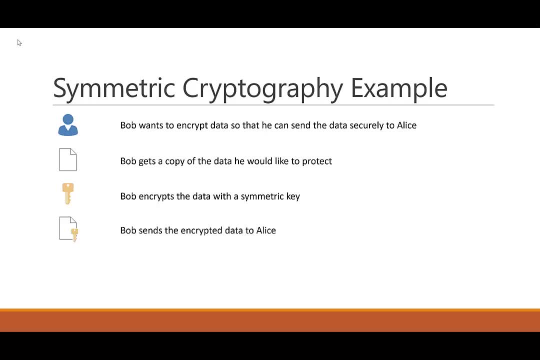 He then gets the symmetric key and then encrypts the data with that key. Bob then sends that encrypted data to Alice, And then Alice uses the same key, which she has a copy of, to decrypt that data And then she can now read that data. So that's just a quick example. 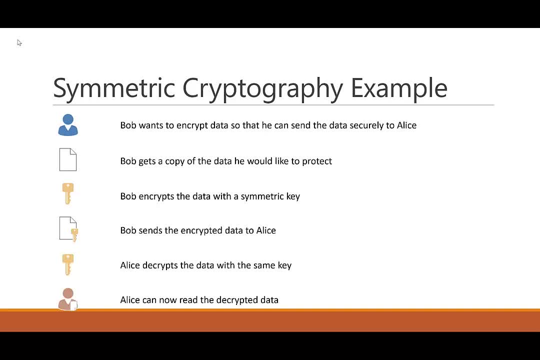 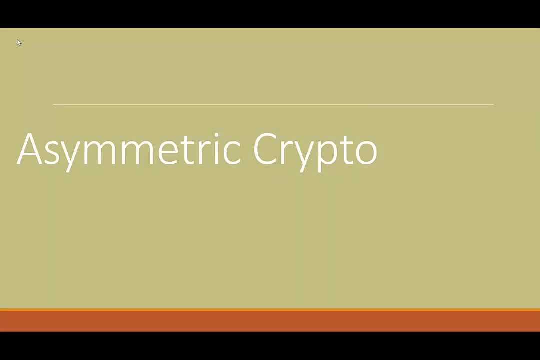 showing how symmetric cryptography works, just to kind of make it maybe a little bit easier to understand. So next we're going to talk about asymmetric cryptography. Asymmetric cryptography is important because it gets into the public and private keys that we're talking about with certificates. So having at least a cursory 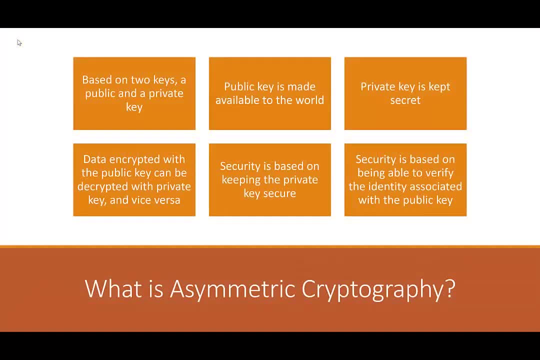 understanding of this is helpful. So asymmetric cryptography is based on two keys. Those two keys are related. right, The public key isn't made available to the world. You can make the public key freely available. You don't have to really be that concerned with securing it. 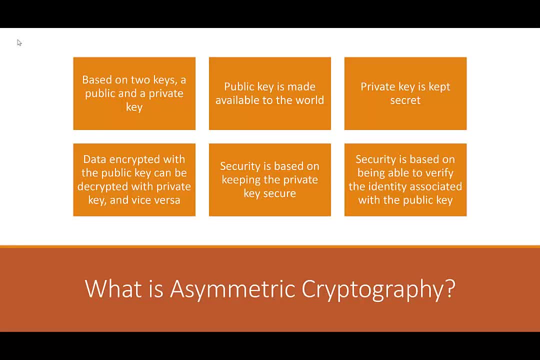 And the private key is kept secret. Now it's very important that you keep that private key secret. That's handled in different ways. Sometimes it's stored in hardware, Sometimes it's protected by software encryption, So there are various ways to do that. 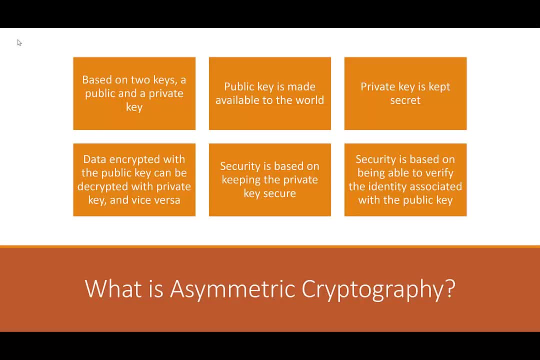 But the main point is that the private key needs to be kept secret because if that key is compromised- and obviously people will be able to compromise data, spoof signatures, that sort of thing- So it's important to keep that private Data encrypted, with the public key can be. 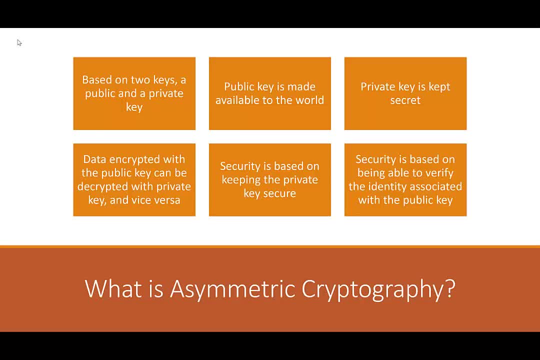 decrypted with the private key and vice versa. So again, if you encrypt something with the private key, it can be decrypted with the public key. if something can be decrypted with the encrypted with the public key, then it can be decrypted with the private key. so there is a relationship in terms. 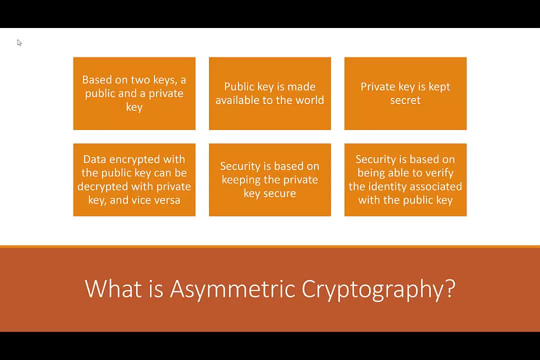 of encryption there and security is based on keeping the private key secure, which we kind of talked about already. and then there isn't a security aspect that's based on able to identify who's associated with that key. right, if we just have keys floating around and we don't really 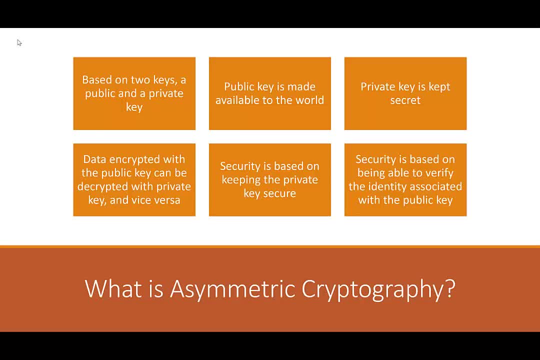 know whose key is whose, it's kind of hard to kind of without that association it it creates some sort of problems for security, and so if you're able to associate an identity with a public key, that's definitely helpful and that that's kind of what certificates do, right, they bind that. 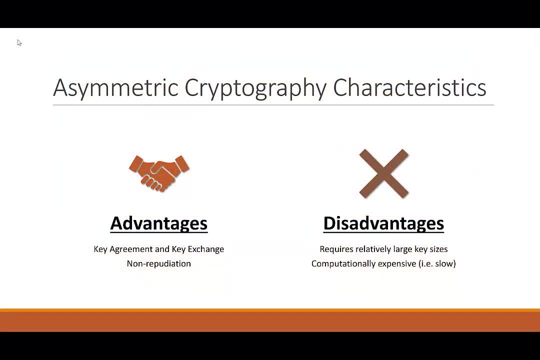 identity to a public key. so here are some characteristics of asymmetric cryptography. so some of the advantages are that um asymmetric cryptography typically supports key agreement, which is basically two individuals coming to an agreement on a same symmetric key, and there's protocols like diffie-hellman that allow users to do that. 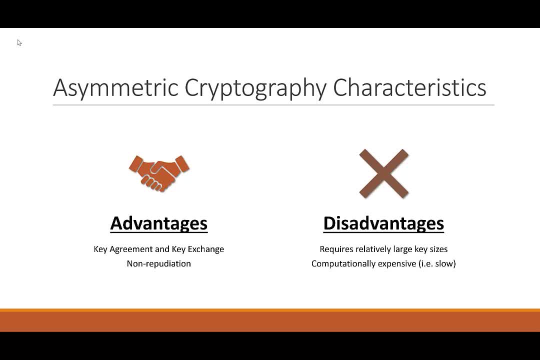 over an insecure network and there's key exchange. key exchange that allows you to basically share a key over insecure medium and then another advantage is non-repudiation. so i gave a quick example earlier: if i send an email to alice and basically if i sign it- which we're going to get to signatures a little bit later on- 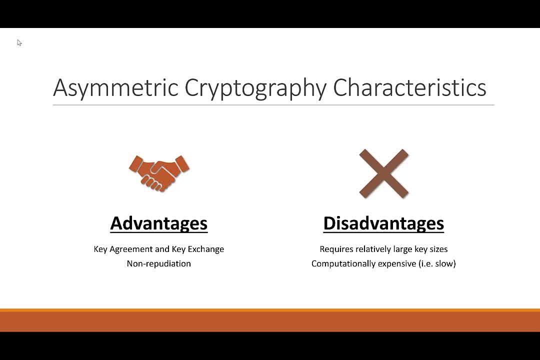 if i sign that email and send it to alice, i can't deny that i send it because through cryptography and hash algorithms, alice can prove that i was the one who sent it. some of the disadvantages are that you'll see um key sizes for asymmetric cryptography are pretty large, like rsa. 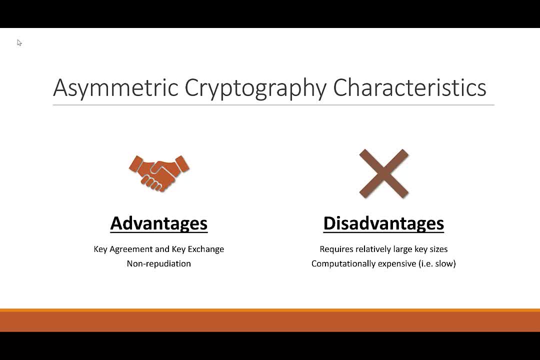 keys are typically around 2k or 20- 48 bit. so that's a large key size compared to asymmetric cryptography. so that's a large key size compared to asymmetric cryptography. where we're talking aes is usually 128 or 256.. there are some elliptic curve cryptography which 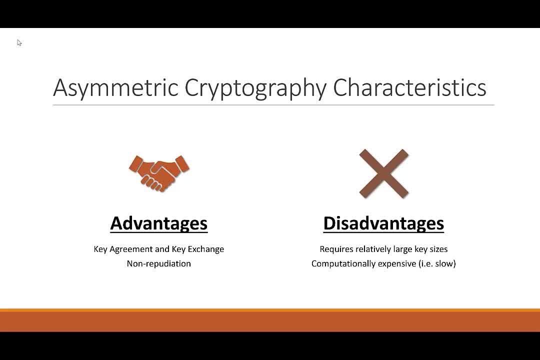 which is more efficient in the sense that it uses smaller keys and it requires less computational power. so there are some protocols, some different protocols, that have been developed to sort of deal with some of those problems, and the other disadvantage is that it's computationally expensive. so this is involved with the factoring of large prime numbers. 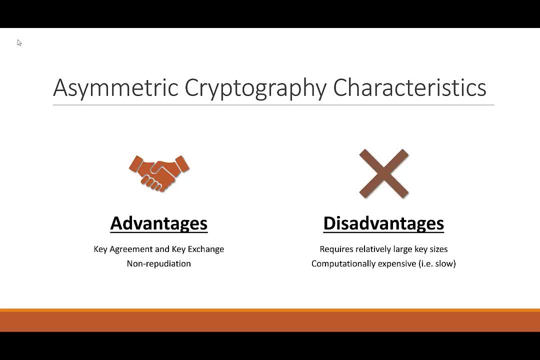 it requires a lot of processing power to create these numbers and and to do all this mathematic work, so it's going to be much slower than a symmetric cryptography. here's, like, some examples of asymmetric ciphers: um, diffie-hellman is a common one we see for a 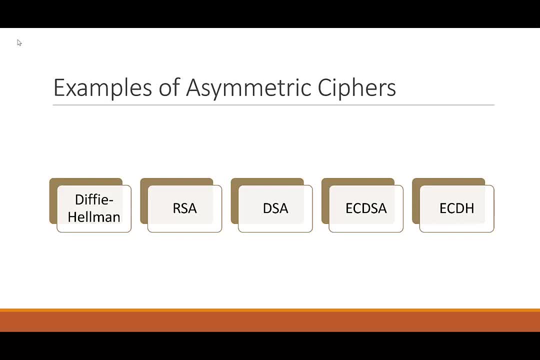 key exchange, and rsa is one we typically see used in certificates, and the last two are elliptic curve, dsa and elliptic curve- defeat hellman. now these are. these are protocols that are going to typically be used in cryptography, and the last two are elliptic curve, dsa and elliptic curve- defeat hellman. now these are. these are protocols that are going to typically be. 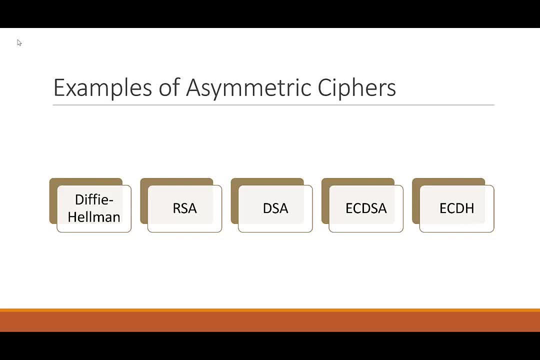 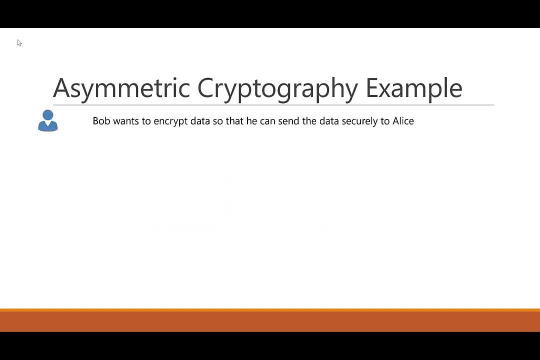 used on devices that have limited processing power. here's an example of asymmetric cryptography. so in this example, bob wants to encrypt data so they can send the data securely to alice. so bob retrieves a copy of the data that he would like to protect, and then he must retrieve a copy of alice's public key. so the question is: 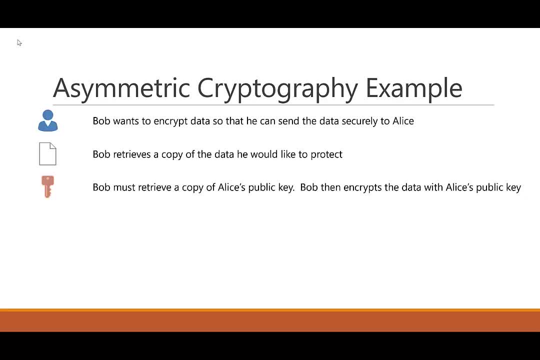 where does he get that public key so it may be stored in different places? of course this is the bag for Esther whovale public key and then, if he liked the content, he'll probably retrieve that public key as a threat to mrышka. he'll do that. but what does this- that's a typical thing- with? 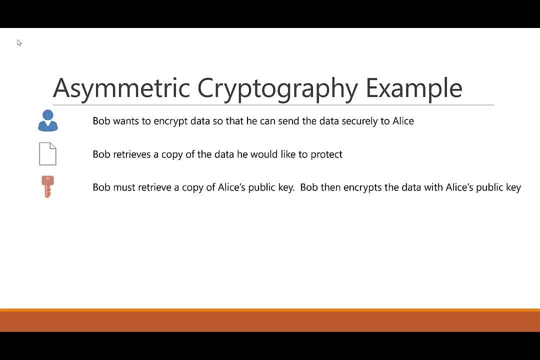 asymmetric cryptography. how do we share that public key? if you go to a website, the public key is on the certificate that's on that website. it was protected by TLS in an enterprise environment. it can be stored in active directory on the user certificate attribute and in exchange, there's certain places where it can be stored. you can have that person's key in their contact and outlook, so there are some different places to get it. so bob retrieved um cleopatra. you see that file. it will be stored. inzza or elliptic curve dsa. 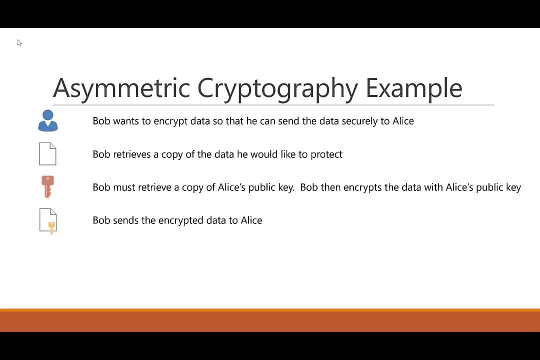 device which is open source. so that's the face, Pretorius, which is the open sourcejaz nichts. here you see, the becomes, with multiplicity already set up, retrieves the key and then he, with that key, he encrypts the data, encrypts the data with Alice's public key. in real world it wouldn't necessarily be used in. 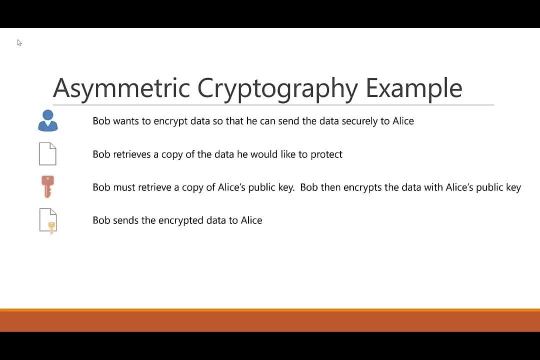 asymmetric cryptography for bulk encryption. but just to look, just for this illustration here we're just gonna say that Bob actually does the bulk encryption with Alice's public key. Bob then sends the encrypted data Alice to Alice and then Alice decrypts the data with her private key, which only she has. 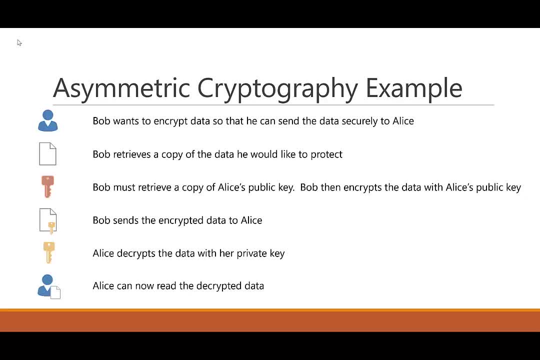 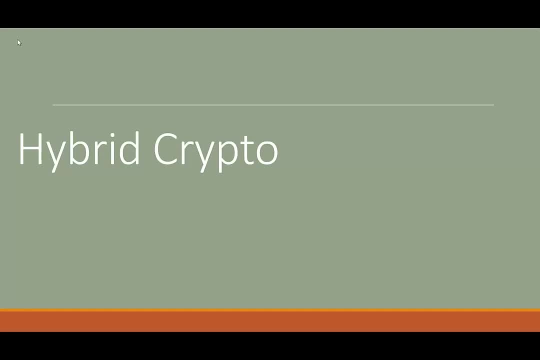 access to, and then Alice can now read the decrypted data and she can access it. so hybrid cryptography cryptography is just- there's other names for it- but this is an example of taking a two types of cryptography and creating sort of a better solution, right? so the use of two crypto systems for a complete crypto. 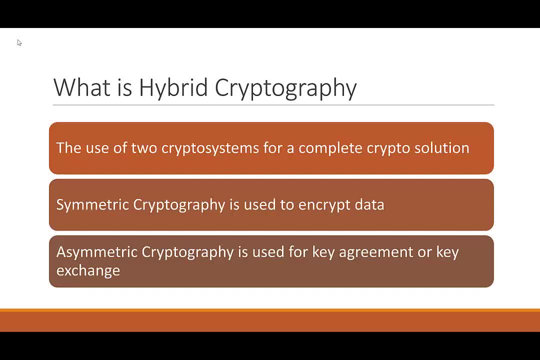 solution. symmetric cryptography is used to encrypt data or do bulk encryption, and asymmetric cryptography is used for key-agreement encryption or key exchange. so we see, when we use these two things together, we get sort of the advantages of each. so we have: we got the speed and smaller key sizes that 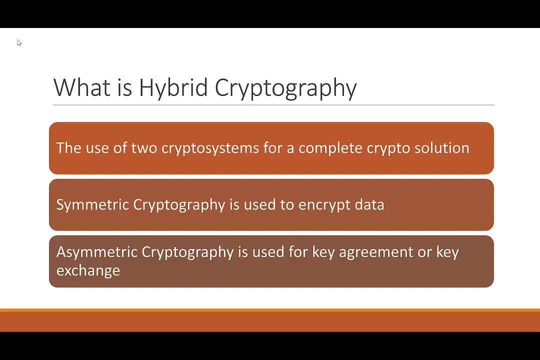 symmetric cryptography has, as well as the lower computational overhead compared to asymmetric cryptography, and then, with the asymmetric cryptography, have a way to exchange these symmetric keys, to either exchange them or come up with key agreement. and there's some other things we can do and we'll see. 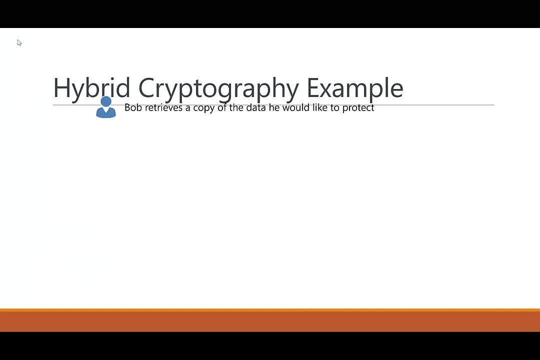 some of these other things a little bit later. so here's an example of hybrid cryptography. so Bob retrieves a copy of the data he would like to protect. Bob creates a symmetric key. again, this is the same key that's going to be used for encryption and decryption. Bob encrypts the data with the best. that same. 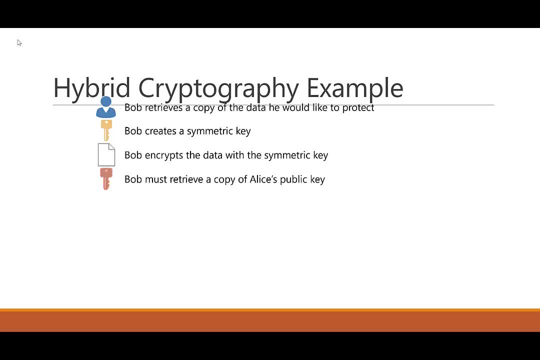 symmetric key that he just created. then Bob goes and retrieves a copy of Alice's public key again. he may get that from different places. Bob then encrypts that symmetric key with Alice's public key. so again the data is encrypted with the symmetric key and in this example the 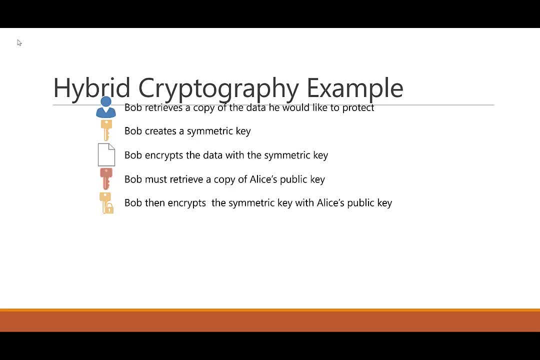 symmetric key is encrypted with the asymmetric key, if that makes sense. so Bob sends all this information over to Alice and then Alice basically decrypts the symmetric key with her private key, which only she has access to, and she now has access to the symmetric key which you can use to go ahead and decrypt the. 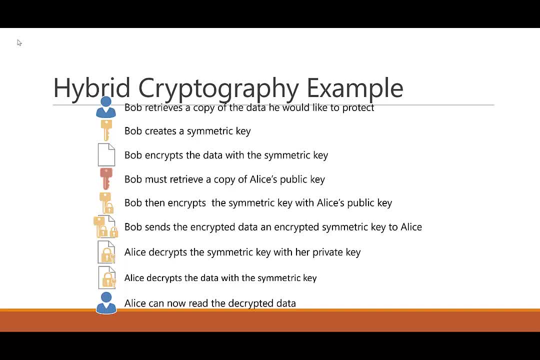 data and then Alice can read it to the crypt of data. so this is one way in which both of these symmetric and asymmetric cryptography can be used together. obviously, in real world applications things may differ little or slightly here, but just to give you the general idea of how this may. 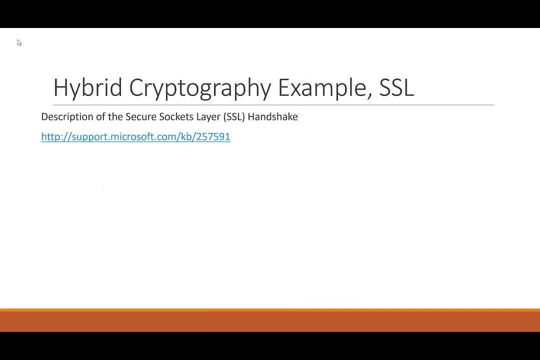 work is the purpose of this example. SSL is an example of hybrid cryptography, where both symmetric and asymmetric cryptography are used. here's a Microsoft KB that discusses on how the SSL handshake happens and that kind of shows you how the different types of cryptography are used. obviously on 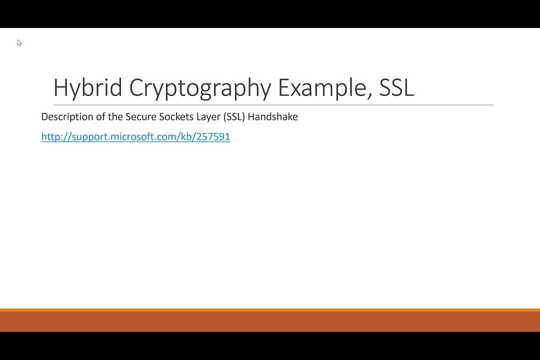 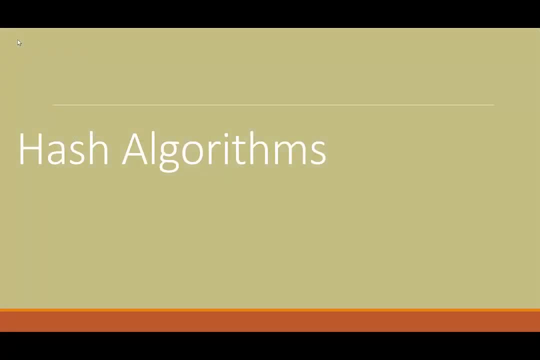 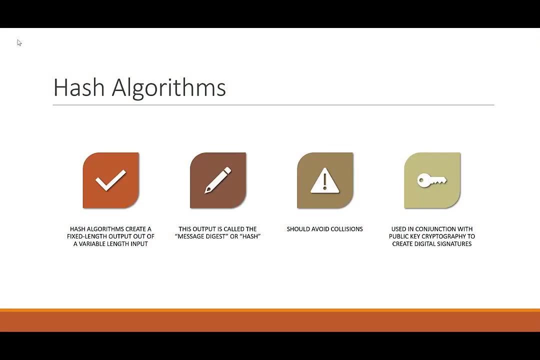 websites. now we use what's called TLS, not SSL. a lot of people still refer to TLS as a SSL, but just be aware that there is a difference: hash algorithm. so next we're gonna talk about hash algorithm. so hash algorithms create a fixed length output out of a variable length input. so what does that mean? so 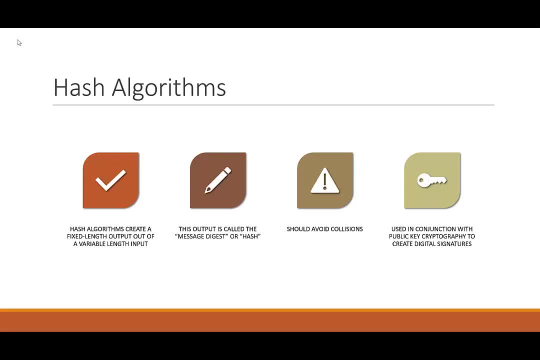 that means I can put- I could put a very large document, let's say hundreds of pages, through a hash algorithm and I will get, let's, I'll get a output of a certain size now, no matter what type of document or material I put to that hash. 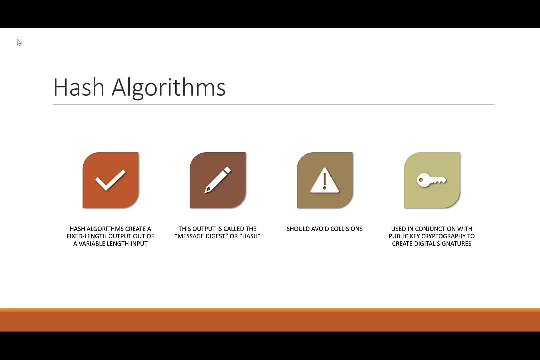 algorithm, I always will get that fixed size, whatever that may be. that output is then called the message digester hash. so those are just two different names for it. the algorithm should avoid collisions. so what does collisions mean? collisions is when you have two different inputs that end up having the same output, so that 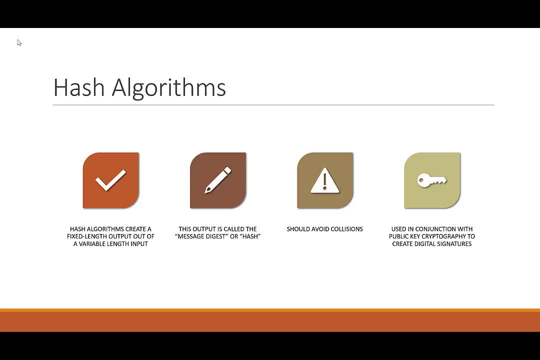 can cause a problem because, especially if you could predict, if you can control what the inputs are and get the same output right, because you could have a, for example, you could have a contract that's signed and then if you are able to alter that contract and still get the same hash. 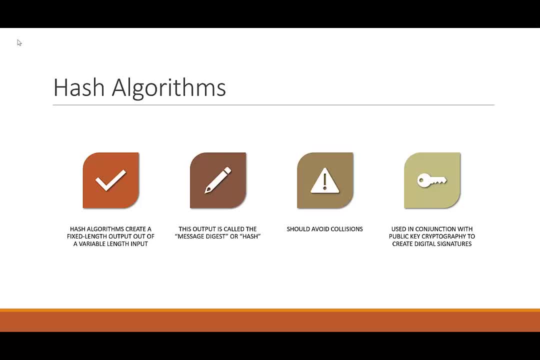 which would result in the same signature. then that could be a problem. so these hash algorithms should avoid collisions. there's been issues found with many of the older protocols. so you know md5 obviously has this issue and shot one has been shown to have this issue. so those are kind of not really. 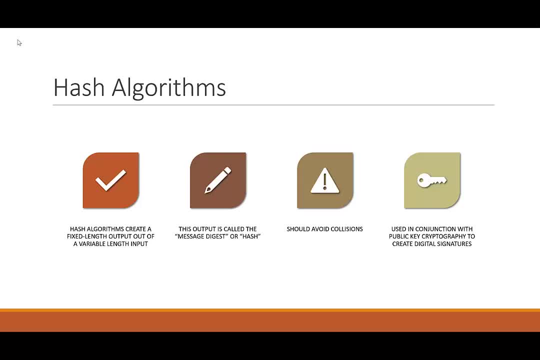 considered secure right now. so these are things that you should not be using. hash algorithms are used in conjunction with public key cryptography to create digital signatures, and we'll see an example of that shortly. here are some examples of hash algorithms again. we have md5 and sha1. 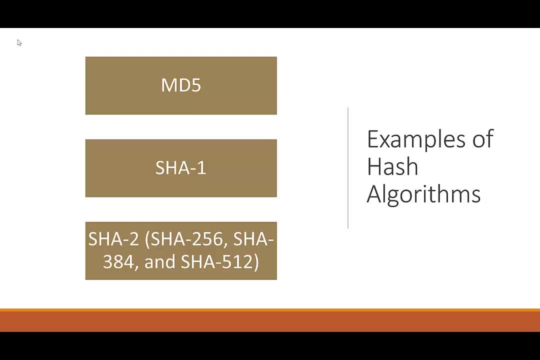 which are sort of insecure at this point. and then we also have what's normally used now in certificates of sha2, and there's, there's, there's, a number of variations of sha2. I think there may be another one in here that's not included, but the ones you typically see are shot 256, shot 384 and shot 512 and real world. 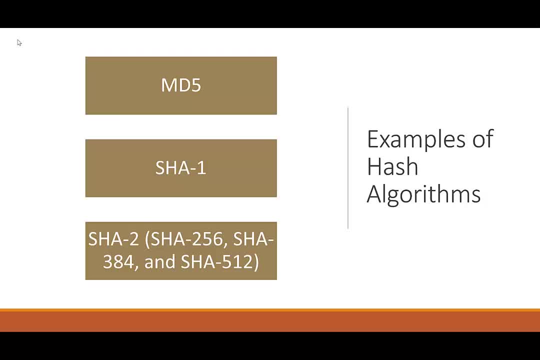 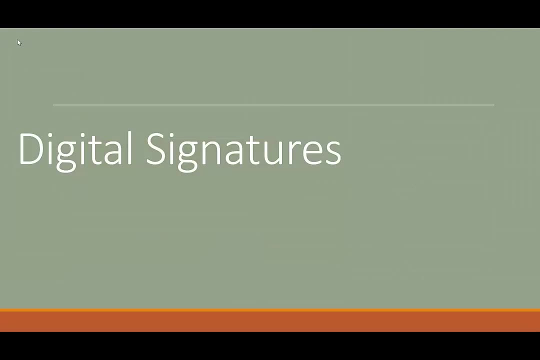 environments. we typically see sha256 typically used, just because there's usually a feeling that that may be more supported between different applications and hardware and services. but there are these three different options that are available to you. so next we're going to talk about digital signatures. digital signatures leverage both asymmetric cryptography. 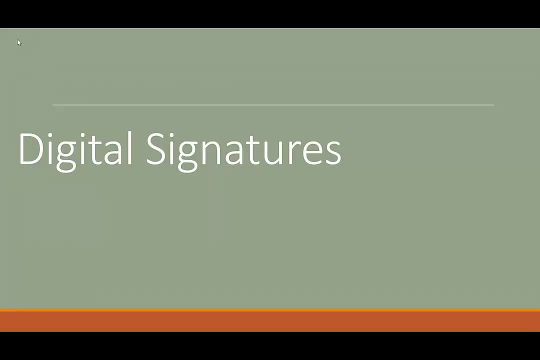 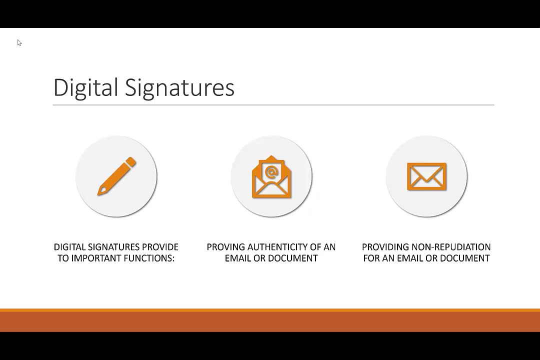 and hash algorithms, and I'll see how that works here in a second. so digital signature. so digital signatures provide two functions, right? so one is they provide authenticity of an email or document, and the other is they provide an authentication of an email or document. so what does authenticity mean? so, 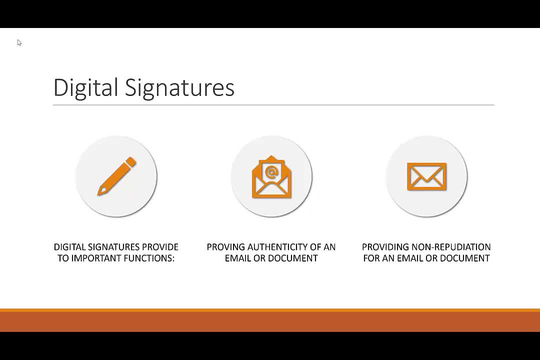 authenticity means. it means basically a couple different things, depending on how you're looking at it, but the main thing I would be thinking about here is that it's a way to prove that the document has not been altered since it's been created, right? so that's kind of an important thing. I- I create a document. I. 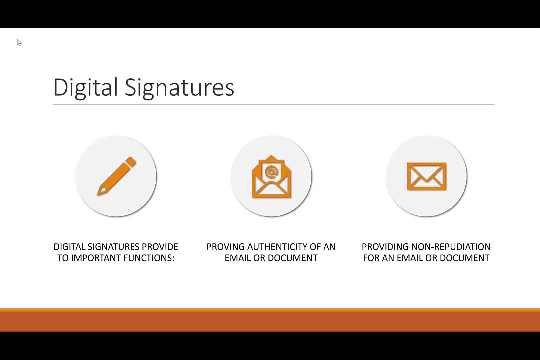 sign it. I send it to Alice, especially if it's a very important document. Alice may want to be able to know that that document has not been altered in transit. so I'm a malicious person, and so digital signatures provide that capability. and then digital signatures can also provide non repudiation for an email or document. 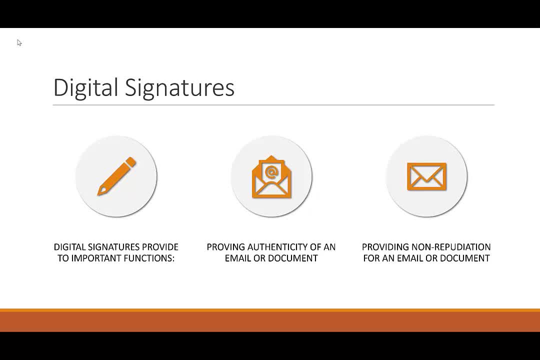 and kind of like we've talked about a couple times already. basically, the idea is, if I send an email to Alice and I sign it, I can't deny that I sent that email because through the digital signature, she can prove that it was signed by me. so these are some of the capabilities or or features that are. 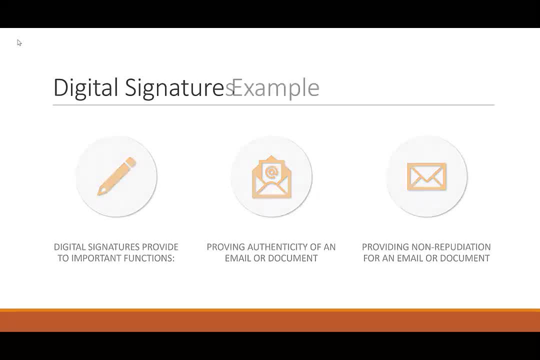 provided by digital signatures. so digital signatures can provide a lot of information and information that I need to be able to use in my digital signatures. so here's an example of a digital signature. so in this example, Bob has a document that he would like to sign, so it's just a Word document for 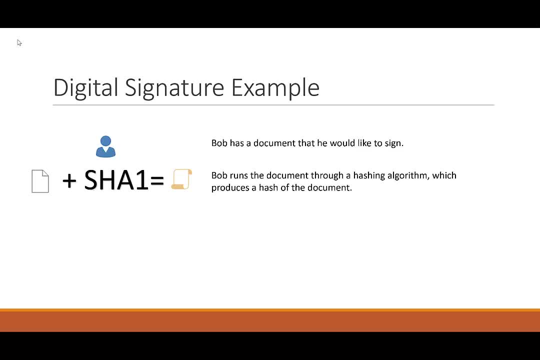 the sake of this discussion. Bob then takes that document and runs it to a hash algorithm. we talked about SHA-1 being insecure, but this is just for the purpose of illustrating this. it's not that important. this is mainly just to understand the process. so Bob takes the document and he basically runs it to a 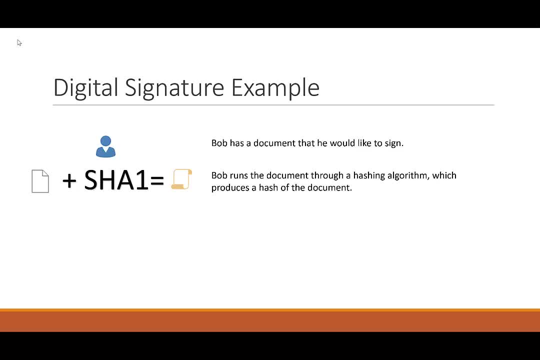 hash algorithm and he gets his hash or message digest right, a fixed length output that should be, you know, unique between different things that could be put through the process. so, anyways, he ends up with his message digester hash. Bob then takes that hash and encrypts that hash with his private key, creating 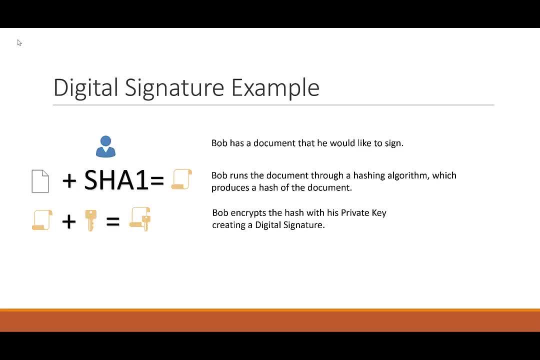 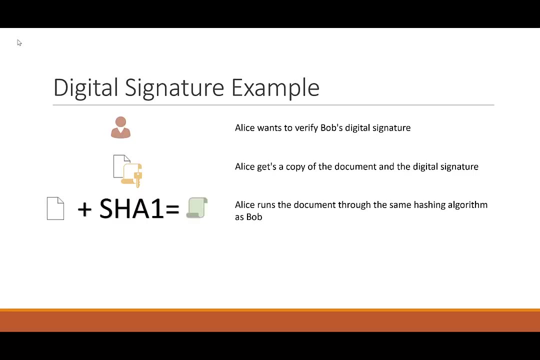 a digital signature. so now he has this digital signature of the document. so he has a document and he has the digital signature. so he sends that document along with the digital signature to Alice. so Alice gets a copy of the document in the digital signature and then Alice is going to go ahead and run. 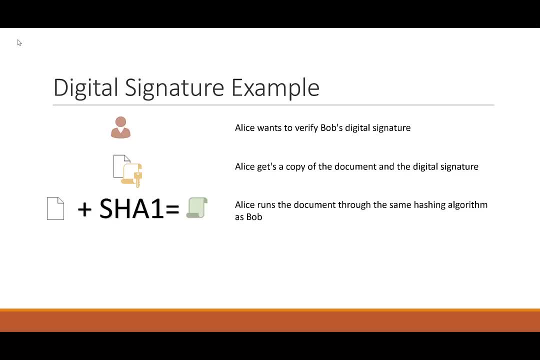 that document to the same hash algorithm algorithm that Bob did. so there's gonna be some metadata in a document that indicates that he used SHA-1. so she's gonna get that metadata, figure out that it's SHA-1 and run the same document through the SHA-1 algorithm and she's gonna get a hash. 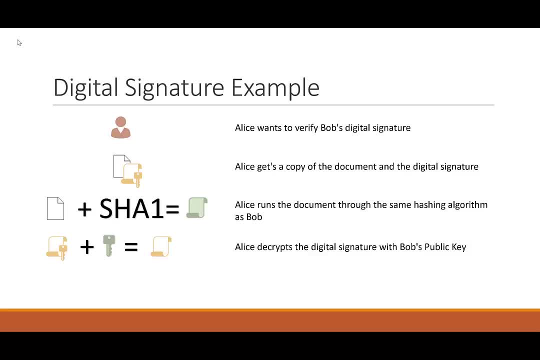 or message digest, as we can refer to either way, and then Alice goes ahead and gets that digital signature and decrypts it with Bob's public key. so remember there's a relationship between the public and private key. since he encrypted something with his private key, it can be decrypted with the public key. 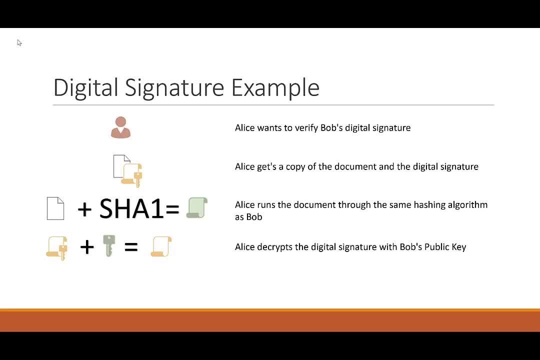 again how she got that public key. that can happen in a different couple different ways. it could, it could likely be included in a certificate that's attached to the signed document. so there's different ways that can be distributed. so at the end of the day, the public key can be used to decrypt the 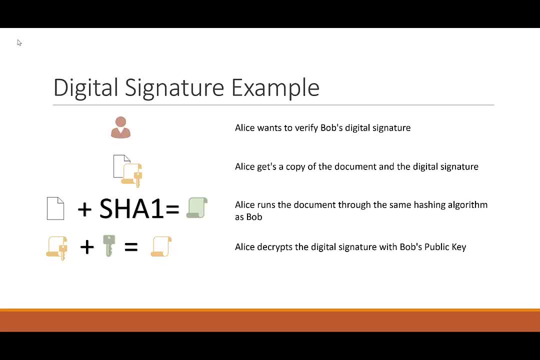 hash and at the end of the, at the end of the situation, Alice has decrypted the digital signature at Bob's public key and then Alice compares the hash she generated, the hash that was decrypted, with Bob's public key. so here's a couple things that we find out. so if the hashes match, we understand, we figure out that. 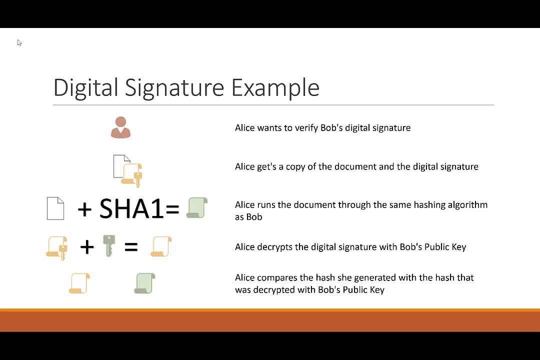 the document hasn't been altered in transit because otherwise the hashes would not match right. if somebody changed some words in the document or anything in the document, the hashes would not line up and then the other hashes would not be able to decrypt it with Bob's public key. she knows through.